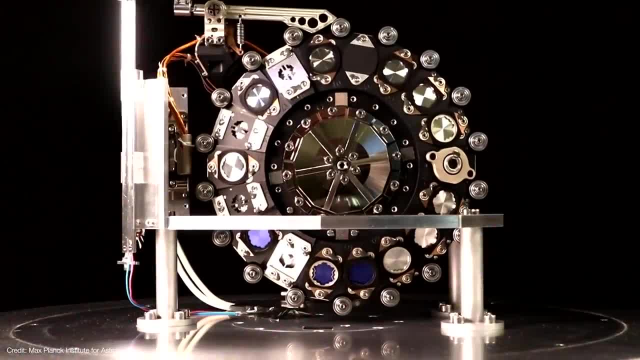 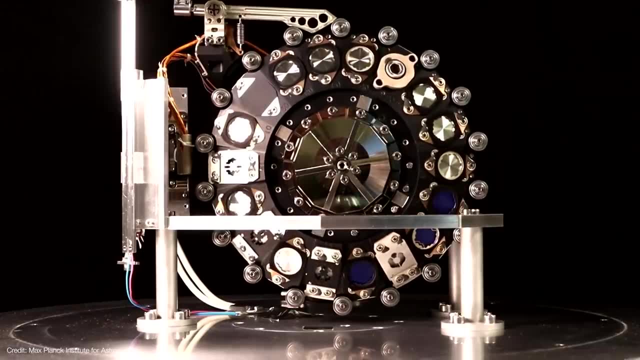 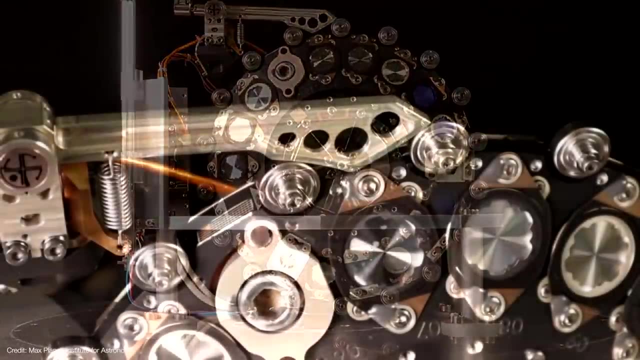 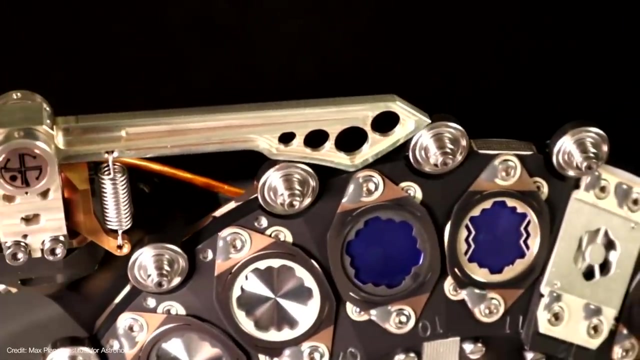 This is a Flight Qualification Model of a filter wheel used on the Mid-Infrared Instrument or MIRI. It looks like a piece of modern techno art, but it's a critical component of what is literally the coolest instrument aboard the James Webb Space Telescope. 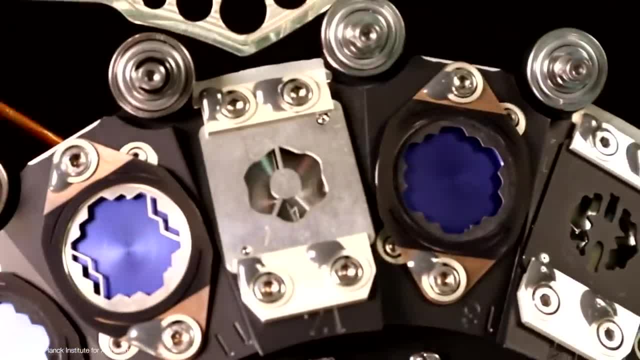 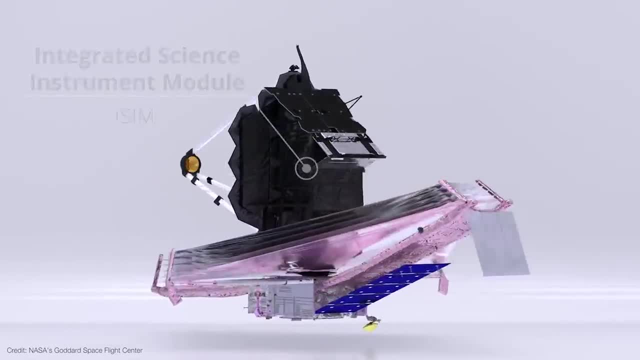 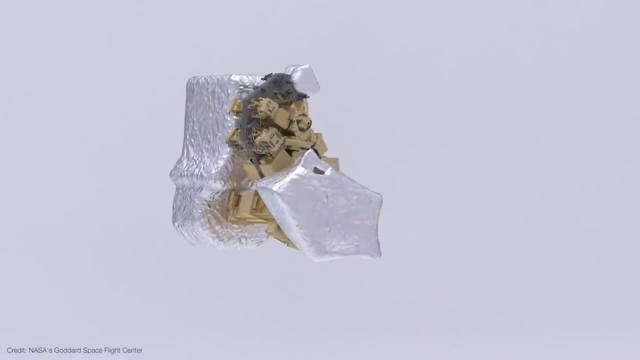 MIRI is one of Webb's four science instruments. They're housed inside the Integrated Science Instrument Module, or ISIM, located behind Webb's primary mirror. Although they weren't designed to be swapped out and replaced like on Hubble, Webb's instruments partially duplicate some of each other's capabilities. 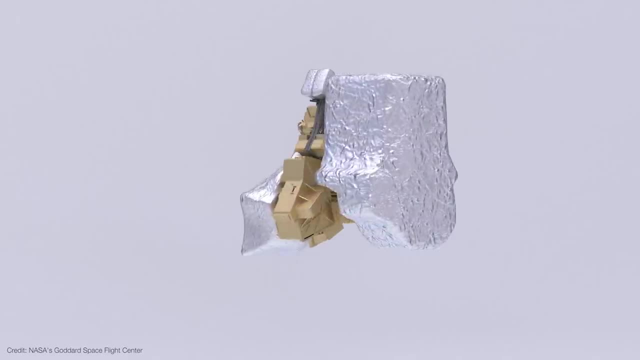 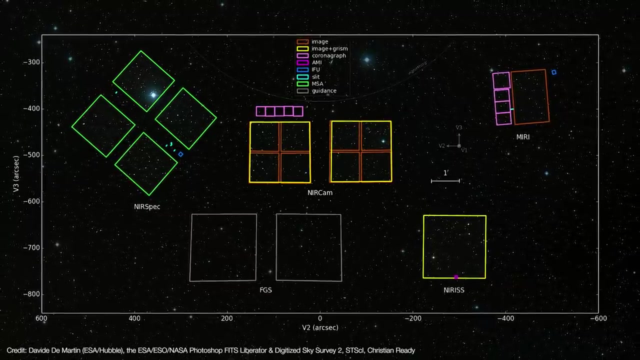 and in some cases, have fully redundant copies of their own hardware on board. The instruments view a portion of Webb's science field of view. This is the part of Webb's total field of view that's optimized for maximum image quality and avoids as much of the stray light as possible. 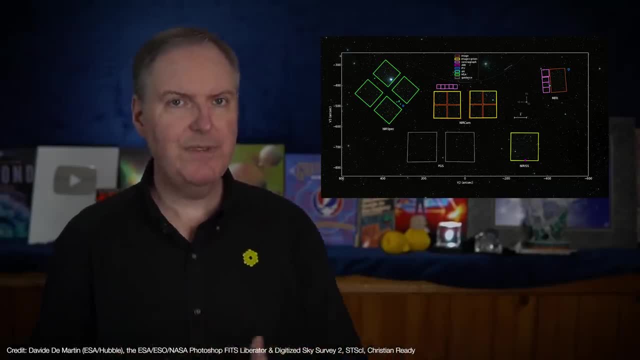 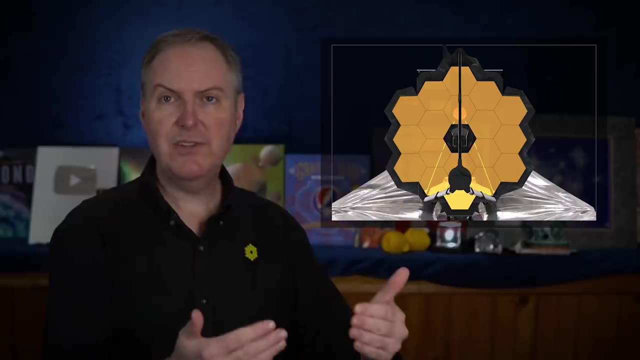 We talked about how Webb deals with stray light in a previous video, but what's important to keep in mind is that all 18 of Webb's mirror segments are contributing to the science field. It's not like any of Webb's mirrors are going unused or anything. 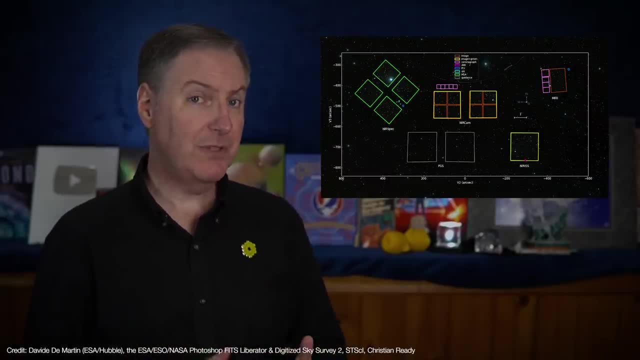 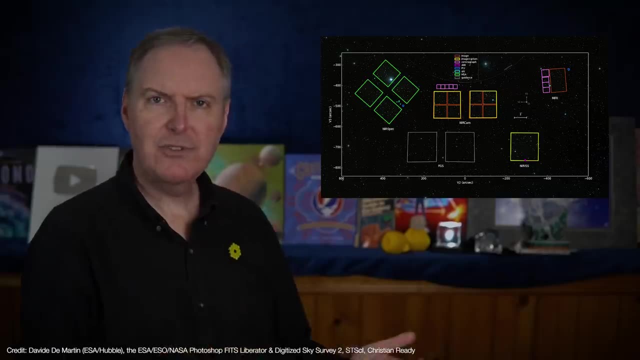 Still, if the instruments are already restricted to a portion of Webb's total field of view, well, why then should we restrict them further? by having them share this field? Why not let each instrument take turns viewing the science field? Well, some telescopes do just that. The Very Large Telescope uses a rotating diagonal mirror to send the field into just the instrument needed for the observation. But rotating mirrors introduce additional complexity and risk. so there's really no reason to take such an approach with Webb unless the science requirements demand it, which they don't. 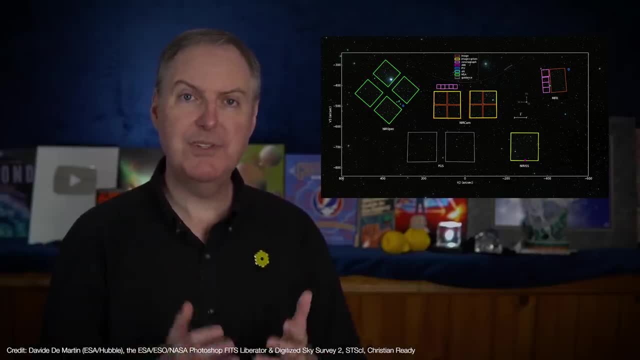 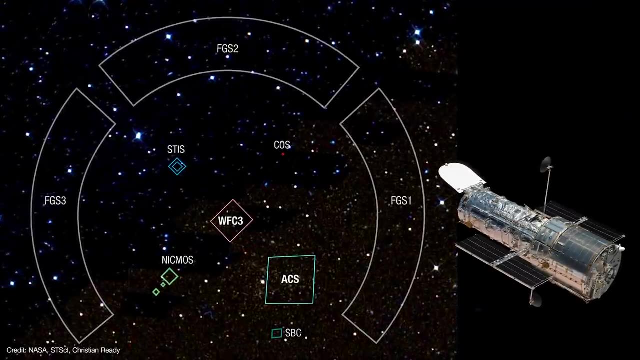 But this approach allows Webb to operate on Webb and to operate multiple instruments at once. It's called parallel observing, which was pioneered with the Hubble Space Telescope in the 1990s, and it's a great way of maximizing science. All of Webb's instruments must be very cold. 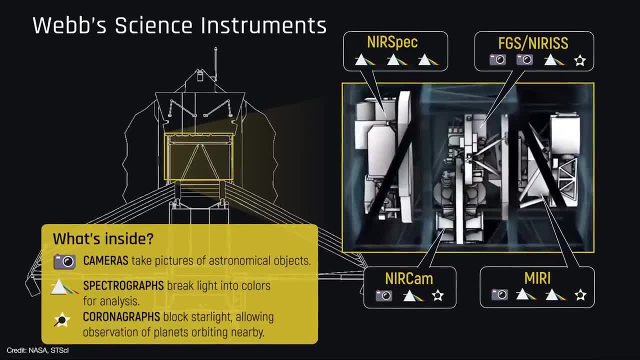 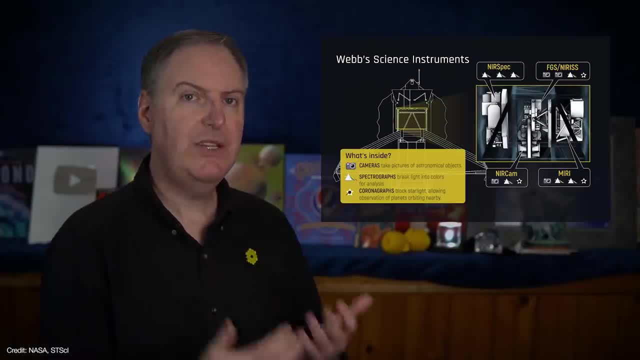 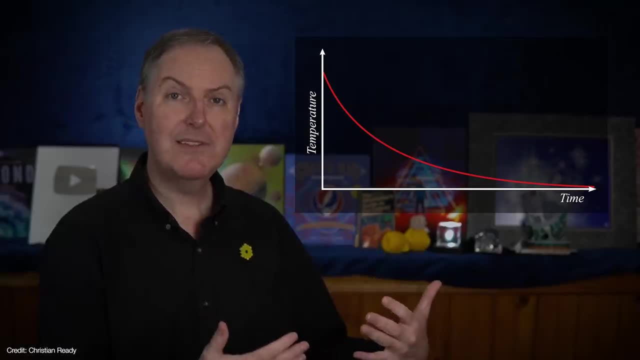 in order to detect faint infrared signals coming from across the universe. The near-infrared instruments alone will need to reach about 30 Kelvin before they can be used. They will need a few months to reach those temperatures, for a couple of reasons. It takes that long to cool because the colder something gets. 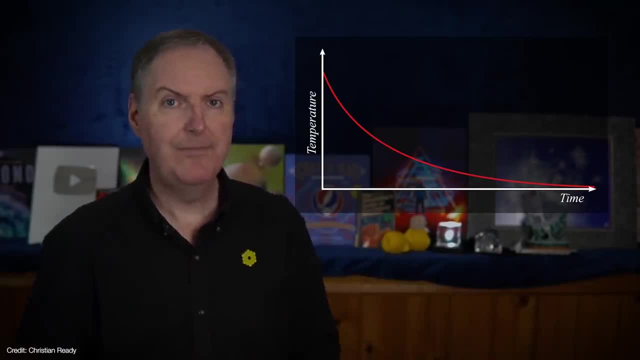 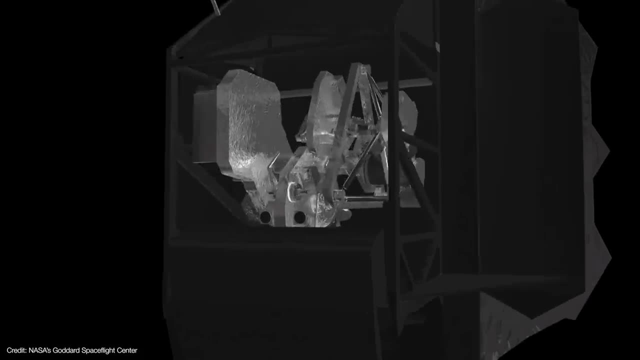 the longer it takes to radiate away its remaining heat. But another reason is that the instruments themselves were kept warm with heaters for about a month after the sunshield was deployed. Now, if you're like me, you're of the strong conviction that 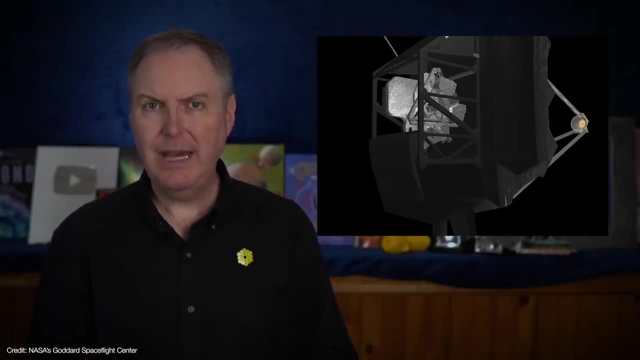 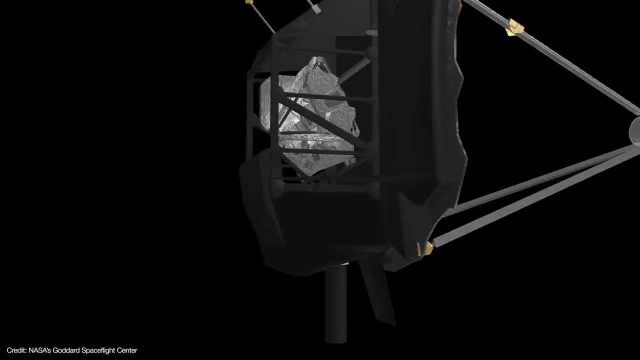 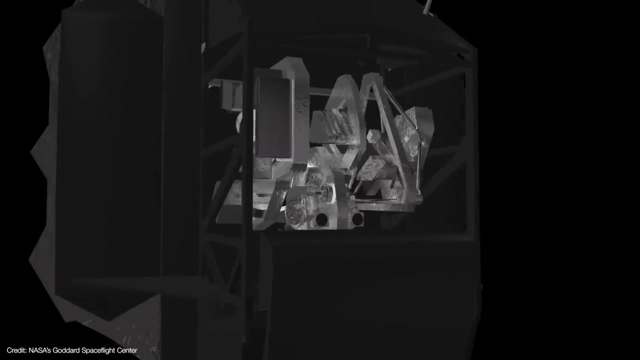 heaters are the wrong device to use when cooling something down. However, the ISIM is made up of carbon fiber, which likely has water vapor trapped within its structures. Once exposed to the vacuum of space, the water vapor starts to outgas. If outgassing water vapor condenses on the instruments' mirrors and electronics. 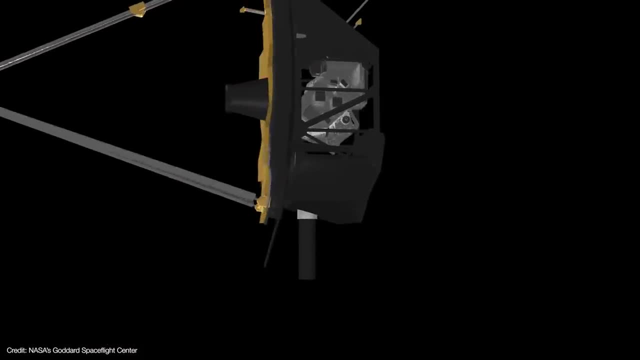 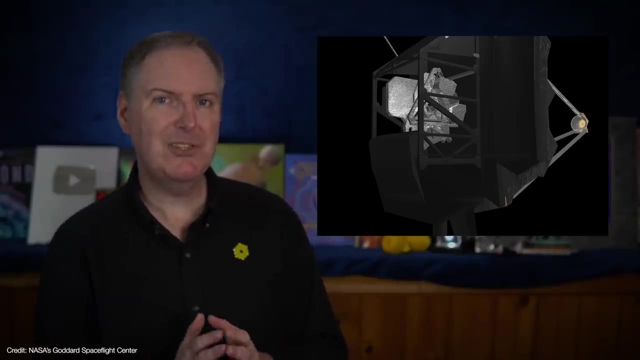 it will quickly freeze into place and probably render the instruments useless, and that's bad. So those heaters kept the instruments just warm enough to prevent contamination as the rest of the ISIM structure cooled. When the ISIM's temperature fell below 140 Kelvin. any remaining moisture was either completely trapped inside the instruments or had already frozen solid onto non-critical surfaces. So even though the sunshield was deployed over a month ago, the instruments are only now finally being allowed to cool down to their operating temperatures. So while we're waiting, let's take a closer look at these instruments. 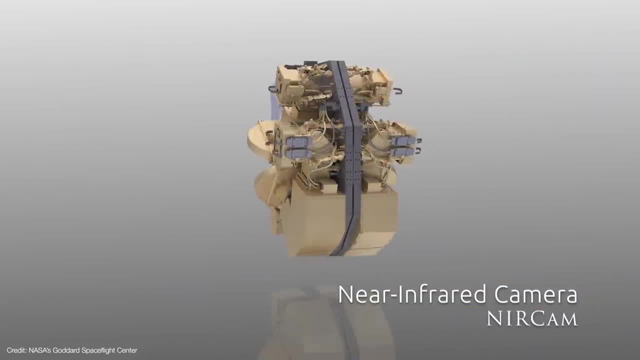 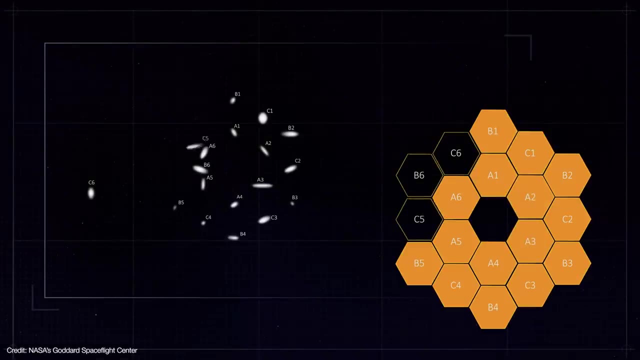 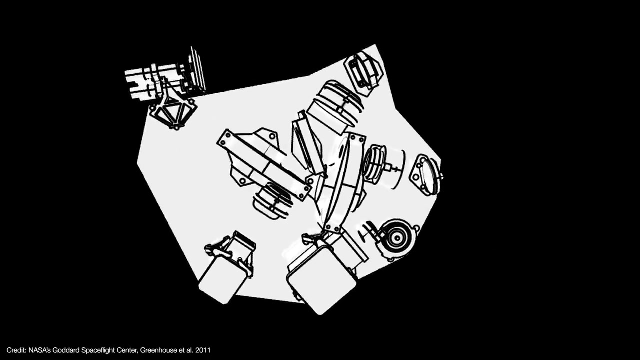 and what they'll show us. First up is the Near Infrared Camera, or NIRCam. This is Webb's workhorse imager that's now being used for the initial mirror alignment process. NIRCam consists of two fully redundant modules that can be used simultaneously. 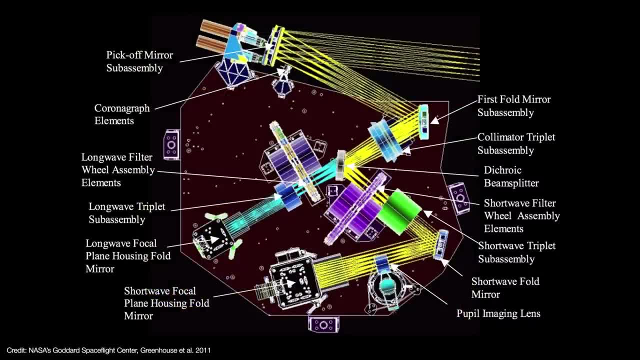 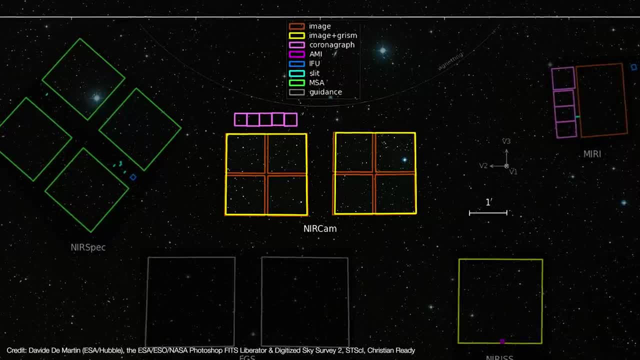 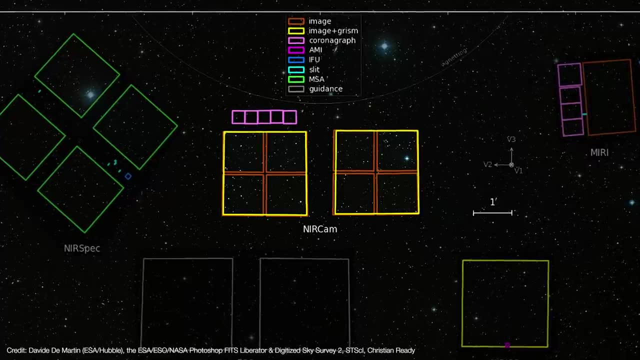 Each module uses a beam splitter to send the light into a pair of short and long wavelength channels. So NIRCam is really two cameras side by side in two completely redundant modules, and each module has two channels for short and long wavelengths, Because it images at shorter wavelengths. 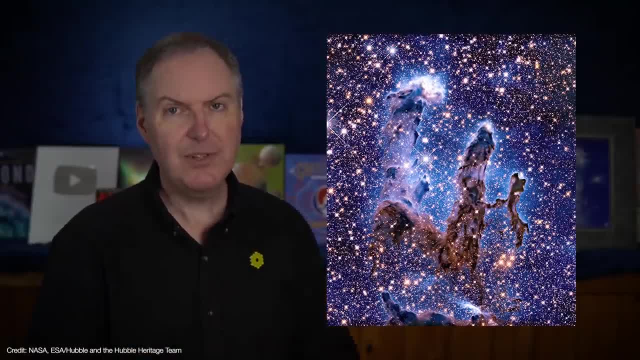 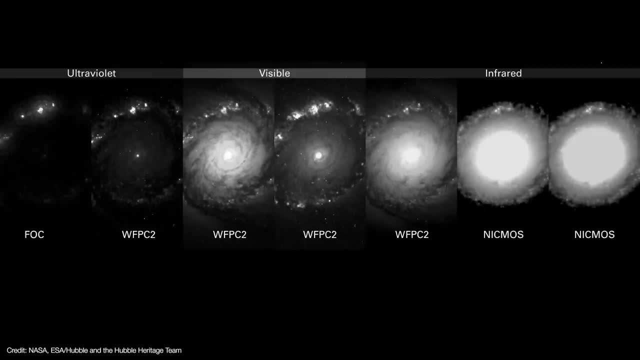 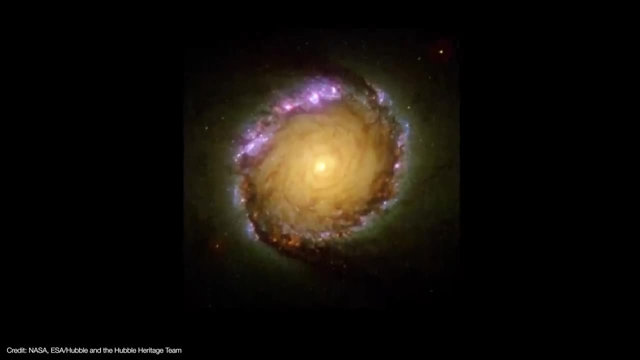 NIRCam will produce Webb's highest resolution images, all of which are grayscale. You see, rather than taking fixed color images, astronomical cameras take multiple images of the same target through different filters. These images can be combined later to produce a color image, And this approach allows the camera to devote 100%. 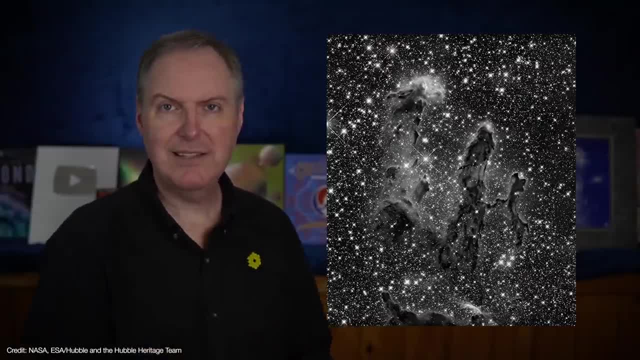 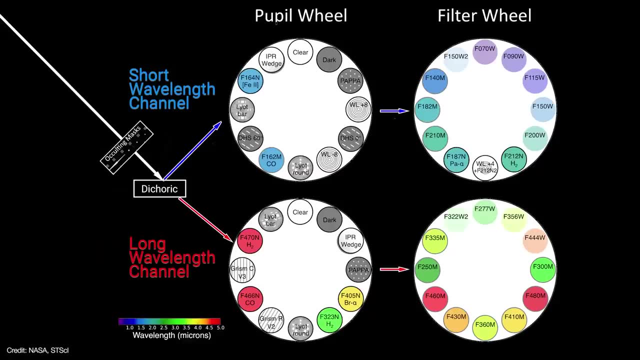 of its sensitivity to just one color at a time, rather than dividing it up among multiple colors simultaneously. To that end, NIRCam uses a pair of pupil and filter wheels in each module, But these wheels allow NIRCam to do more than just take pictures. 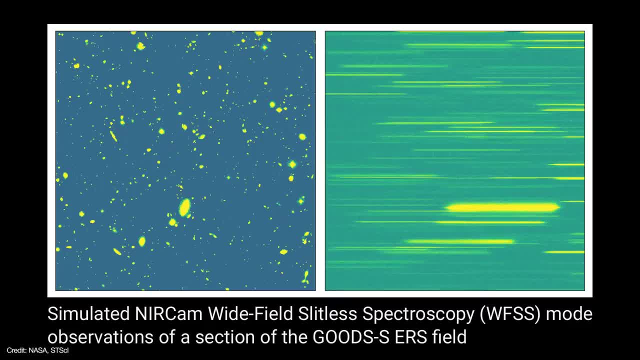 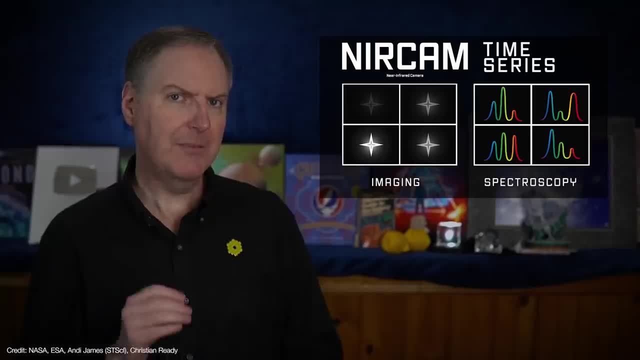 For example, in the wide field spectroscopy mode, light is passed through a prism to create a spectrum of every source in the field. NIRCam can also operate in time series modes as well, And this is where it takes a series of short exposures. 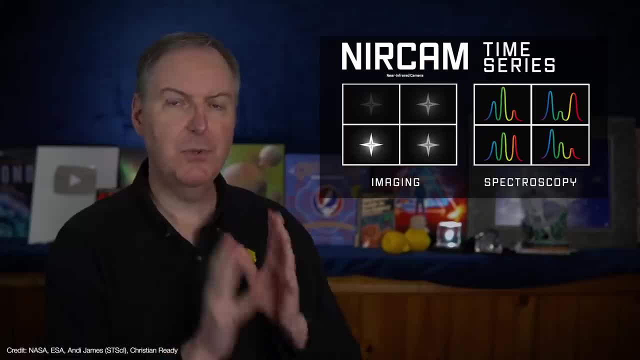 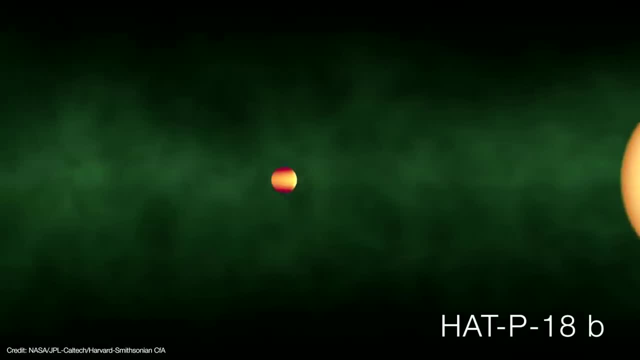 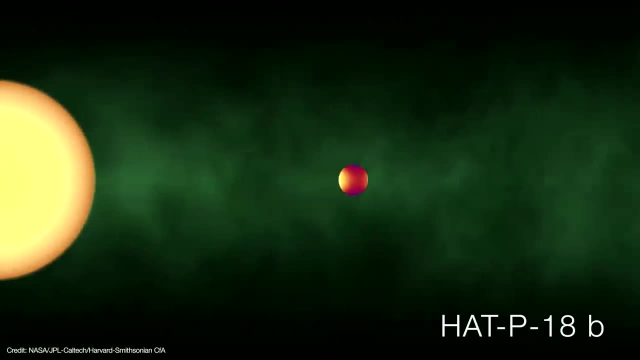 to precisely measure tiny variations in a source's brightness, or even variations in its spectrum. So one early use of time series imaging will be to monitor the exoplanet HAT-P18b as it passes behind its host star, As it does so starlight reflecting off the planet. 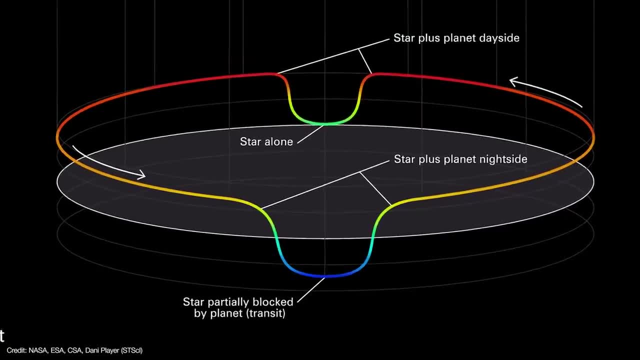 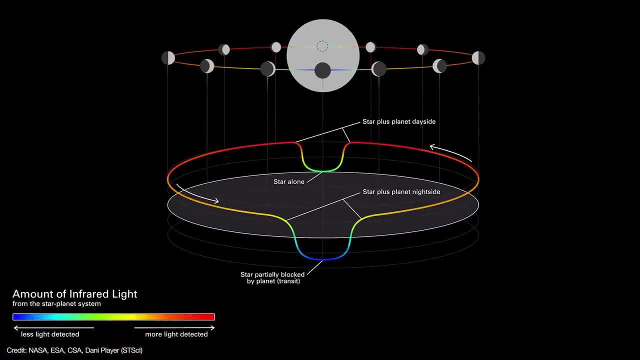 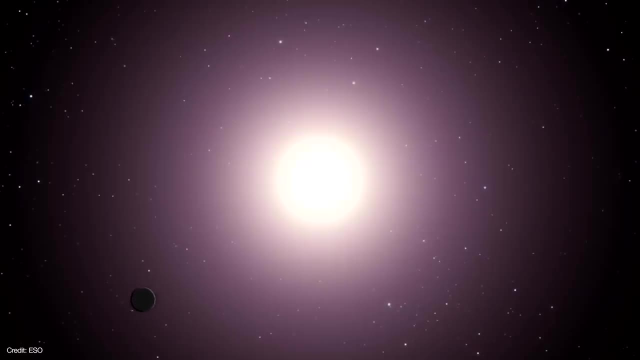 is gradually cut off. The shape of the resulting light curve gives an insight into the density and thermal structure of the planet's atmosphere. Both of NIRCam's modules include an array of coronagraphic masks. These are tiny disks or bars that can block out the light. 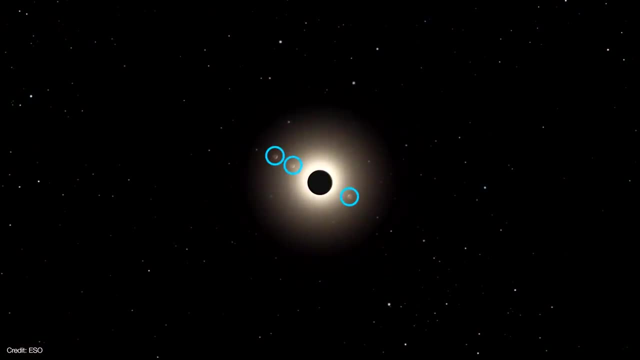 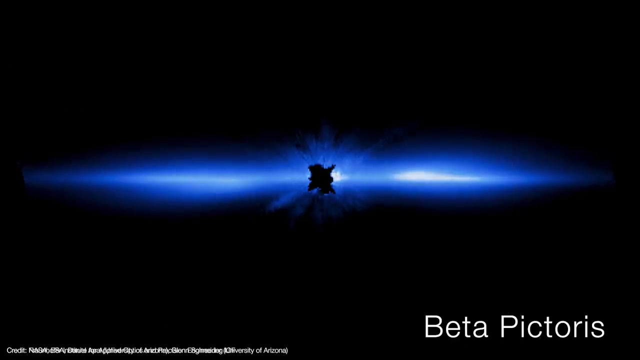 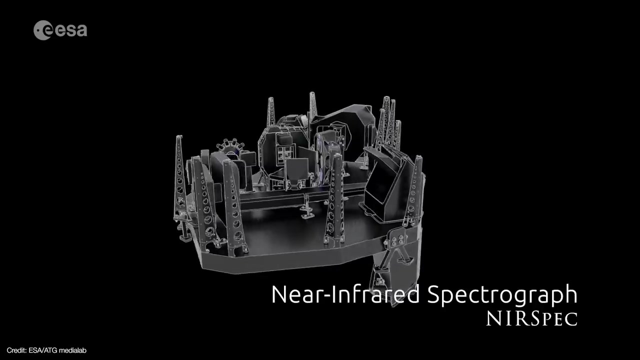 from a bright object to reveal fainter objects next to them. One of its early uses will be to block out the star Beta Pictoris to study its surrounding protoplanetary disk. But if NIRCam is Webb's workhorse camera, NIRSpec is Webb's workhorse spectrograph. 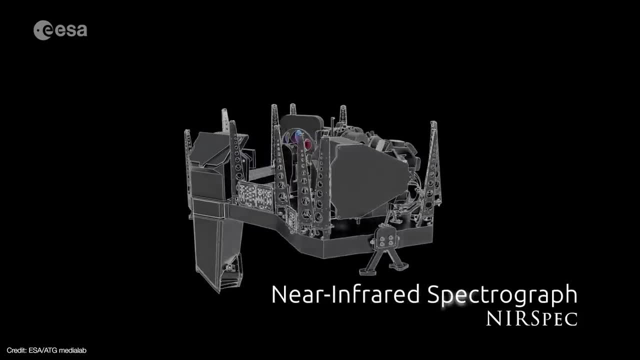 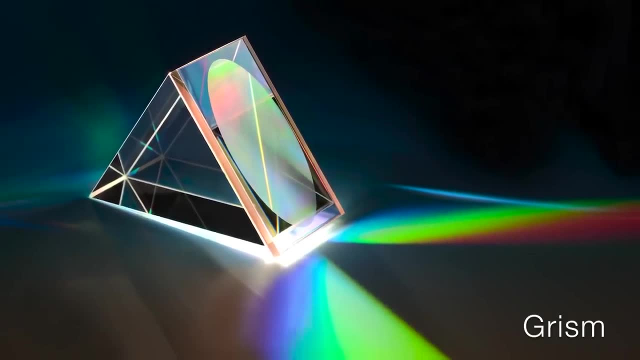 Spectrographs work by passing light through a prism or reflecting it off of a device. In fact, most spectrographs use a combination element called a grism for this very purpose, But NIRSpec carries a fundamental technology that takes spectroscopy to a whole new level. 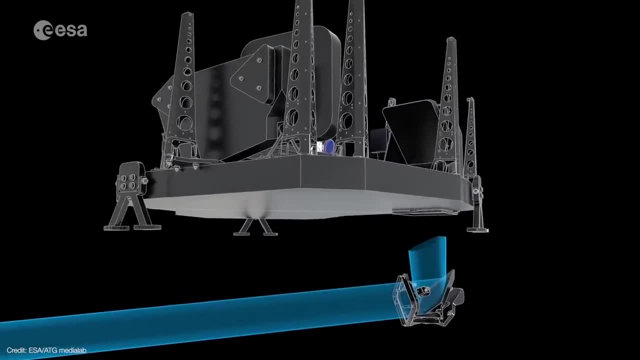 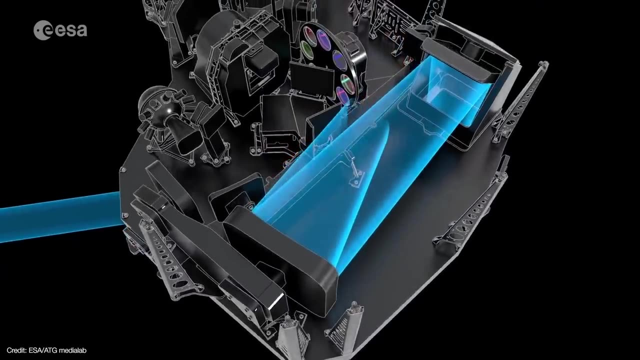 Let me show you how this works. A pick-off mirror sends the light from the telescope's optics into the instrument. The beam is directed to a curved mirror that prepares the image. It's then sent through the filter wheel and then refocused before entering the spectrograph. 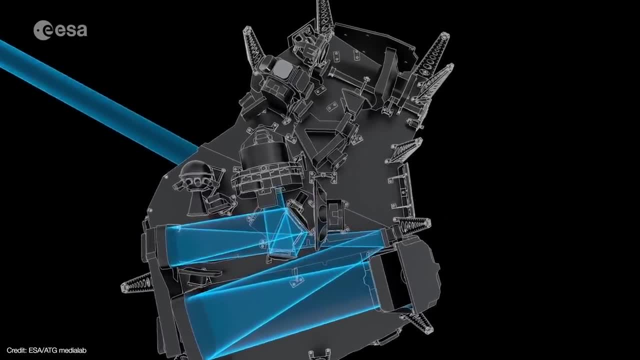 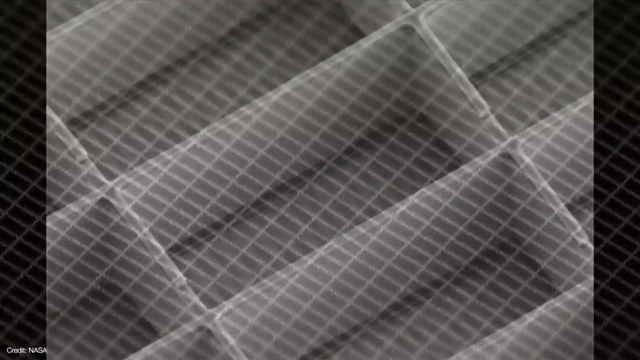 Now here's the amazing part: As it's entering the spectrograph, the image reaches an array of tiny windows called microshutters. Each shutter is only 100 by 200 microns- That's about the thickness of only a few human hairs. 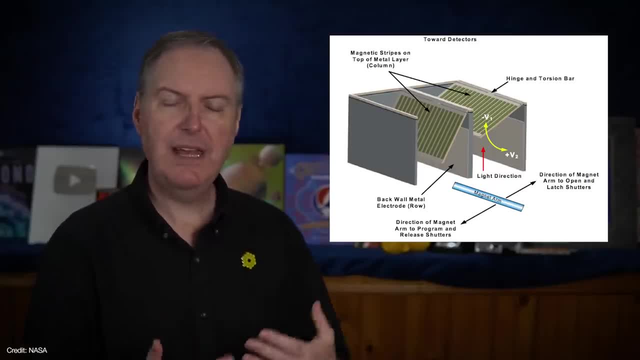 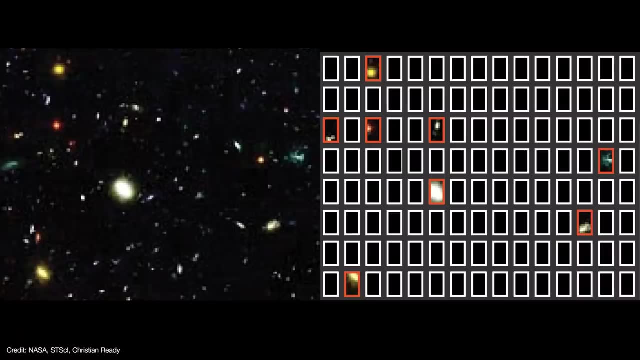 Prior to an observation, preselected shutters are given a small electric charge. A magnetic arm sweeps past and the charged shutters swing open. Open shutters allow light from a particular part of the field to pass through, while the closed shutters block everything else. 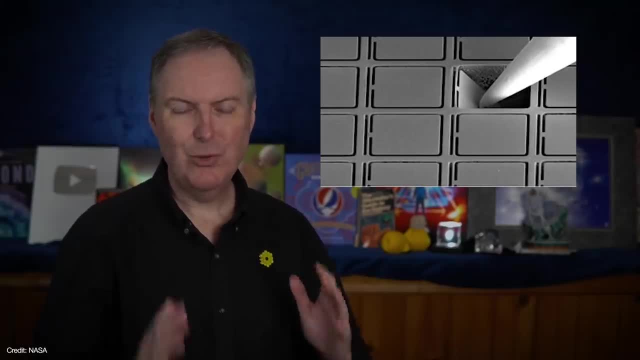 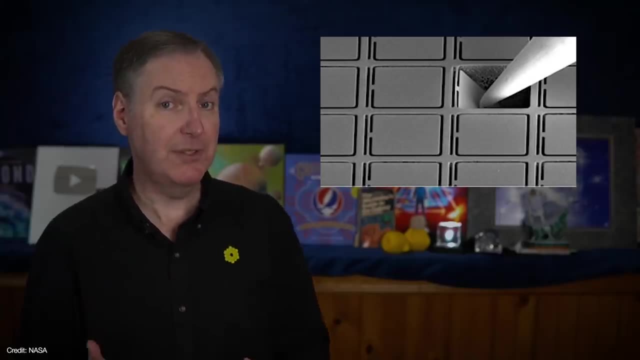 Now, the fact that these tiny shutters can operate at cryogenic temperatures without fatiguing is mind-boggling. They're made of silicon nitride, which was chosen because of its high strength and its resistance to fatigue, And this allows the shutters to be opened and closed again. 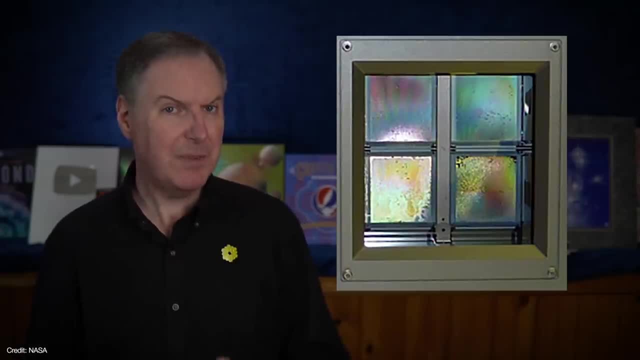 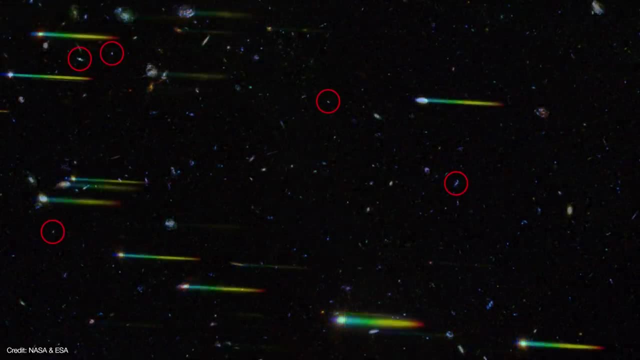 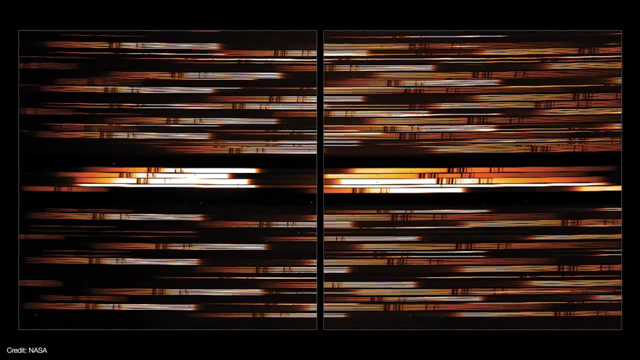 without the risk of breaking off or getting stuck. There's about 250,000 microshutters, so tiny portions of each field can be precisely targeted while blocking everything else, And this allows NIRSpec to take the spectra of up to 100 targets simultaneously. 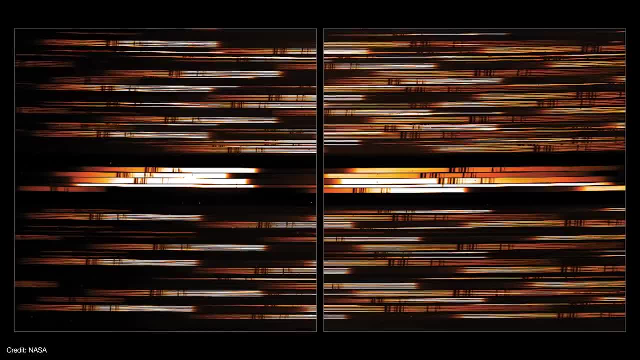 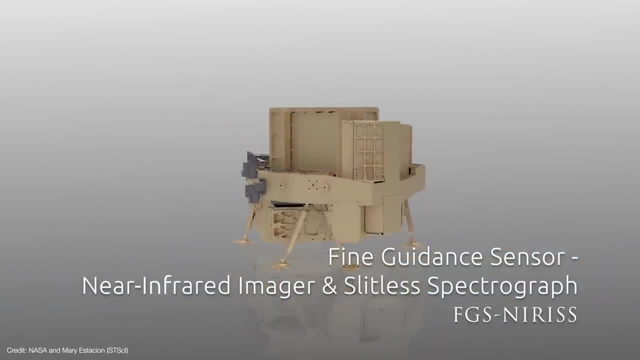 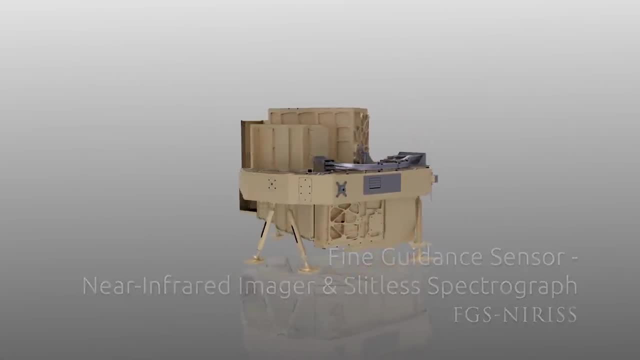 without risking contamination from the background or other objects in the field. Another of Webb's spectrographs is the Near Infrared Imager and Slitless Spectrograph, or NIRIS. It's actually bundled with the Fine Guidance Sensors. FGS, as they're called, is a pair of cameras. 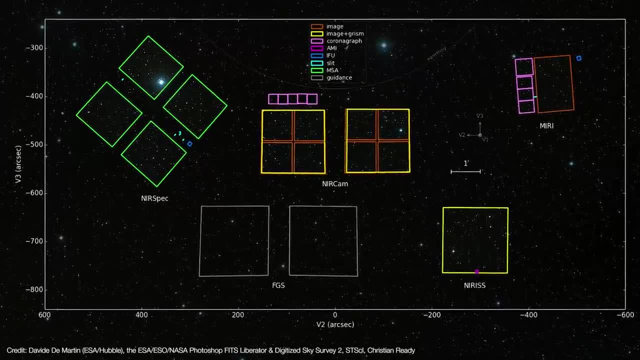 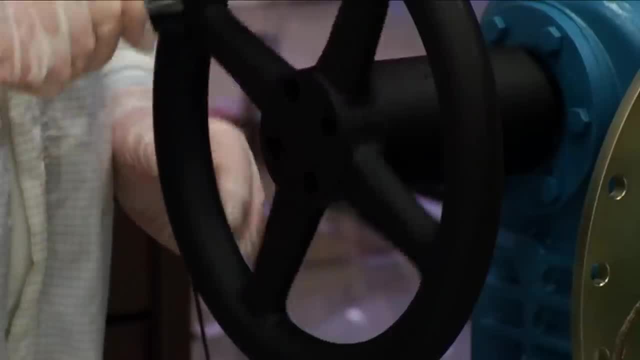 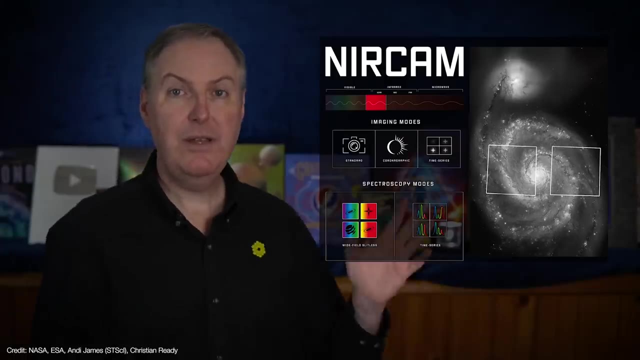 that Webb uses to lock onto guide stars so the telescope can track its science target. That means the FGSs are not available for science, at least for the time being, But the NIRIS side is very much a science instrument Now. earlier we talked about how NIRCam 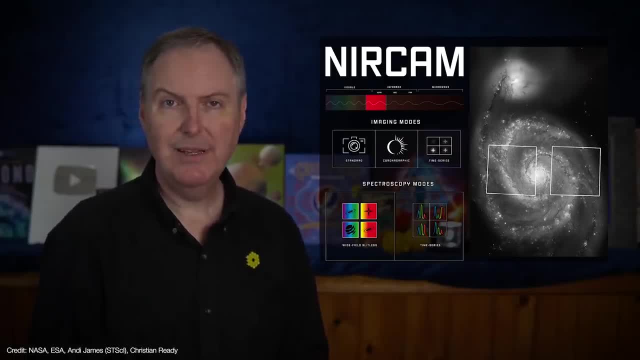 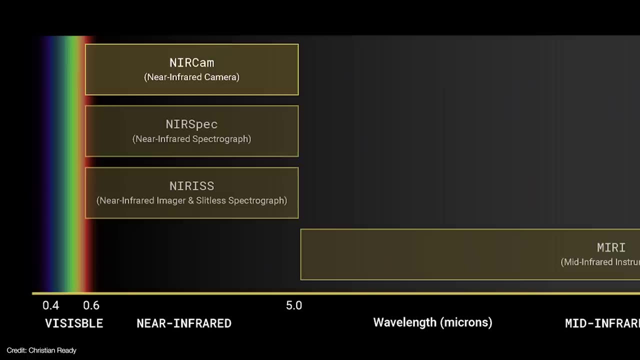 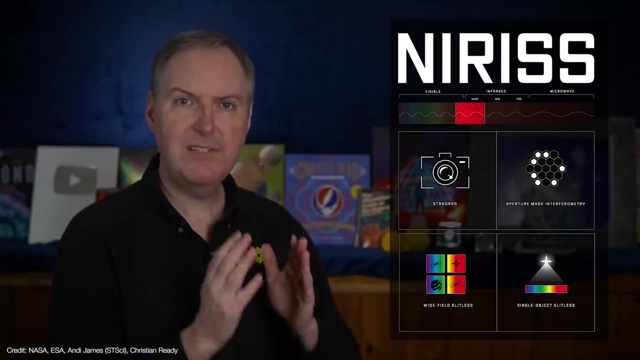 is the main camera with some spectroscopic capability. Well, NIRIS is a high-performance spectrograph with some imaging capability. NIRIS covers the same wavelength range as NIRCam and NIRS, But its spectroscopy modes were designed for two very specific purposes. 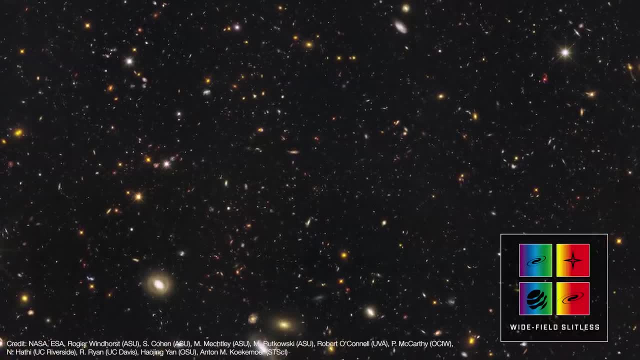 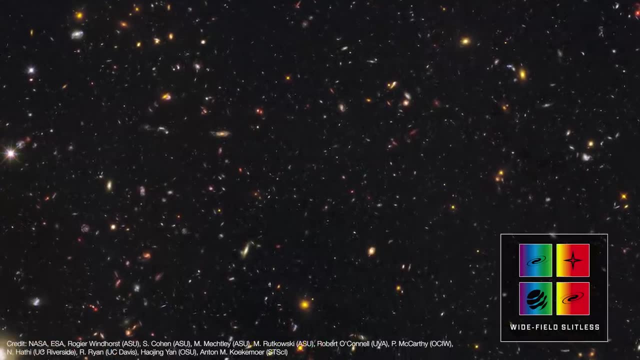 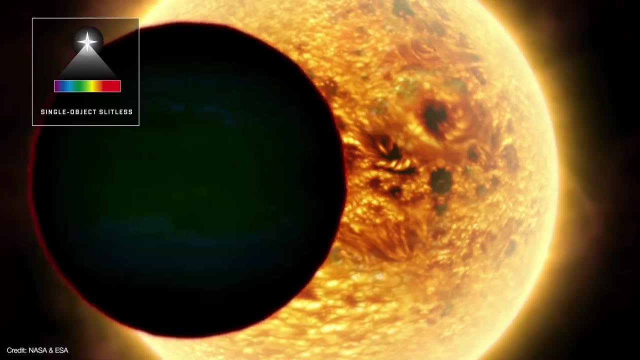 In its wide-field spectroscopy mode, NIRIS is optimized for studying several high redshift galaxies at once, And this allows NIRIS to study star birth in the very first galaxies to form in the universe. In single object mode, NIRIS captures the spectra of exoplanets. 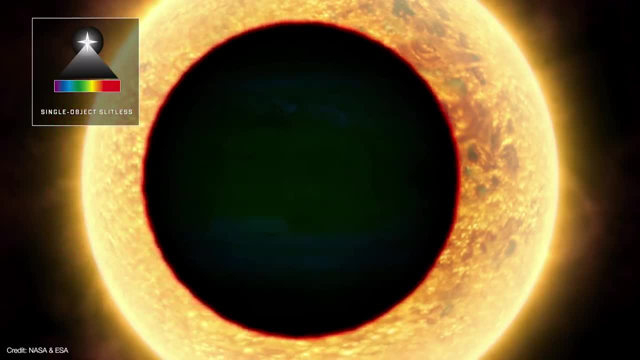 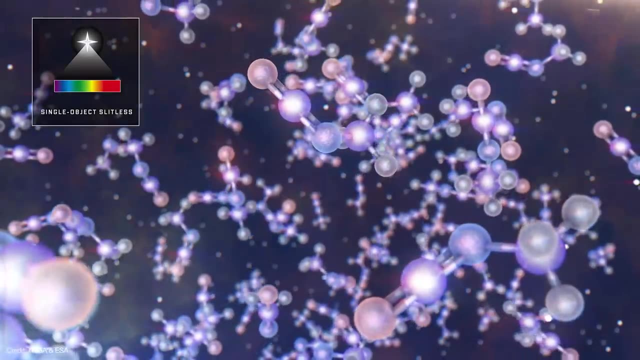 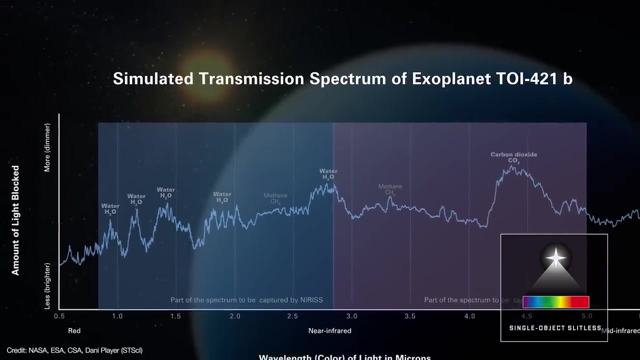 as they transit in front of their host stars. As the planet transits, its atmosphere absorbs certain wavelengths of light while allowing other wavelengths to pass through. By comparing the star's spectrum before and during the transit, the composition of the planet's atmosphere is revealed. 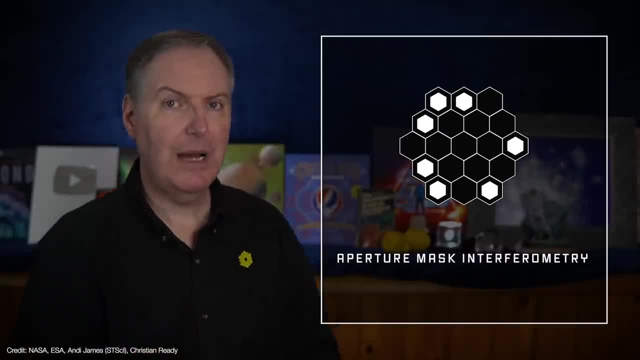 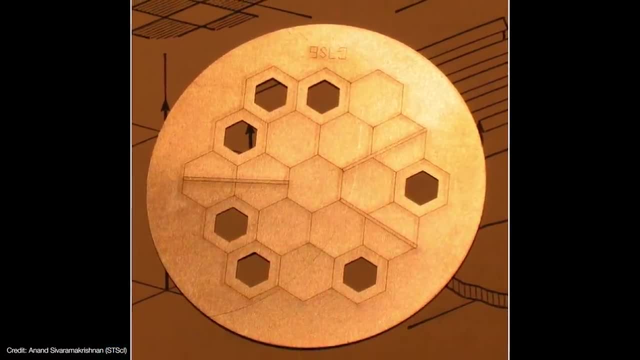 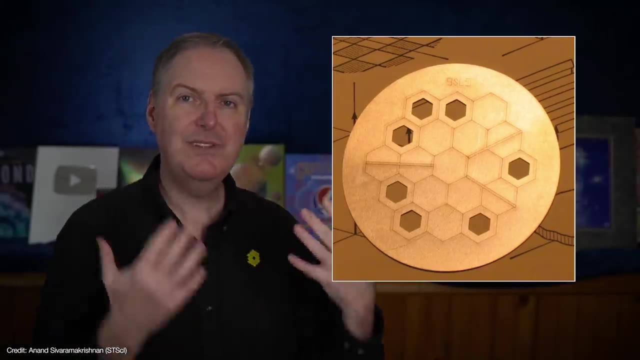 NIRIS also has an Aperture Masking Interferometry mode, or AMI. This mode uses a mask that only allows light from just seven of Webb's mirror segments through. This causes the light waves to interfere with each other and reveal details that would otherwise be too faint to detect. 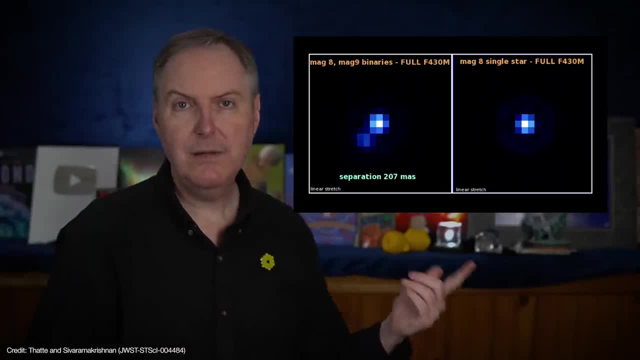 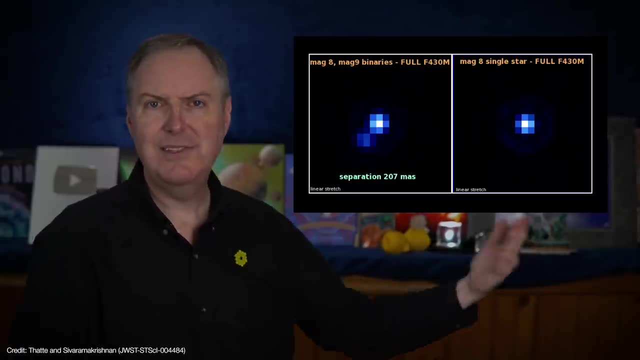 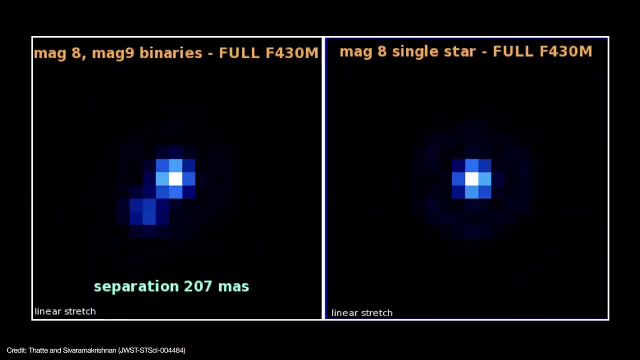 For example, here are simulated NIRIS images of two stars. On the left is what is almost likely a binary star system and on the right is a single reference star. The binary system is too close together to be resolved. They're separated by just 207 thousandths of an arc. second, 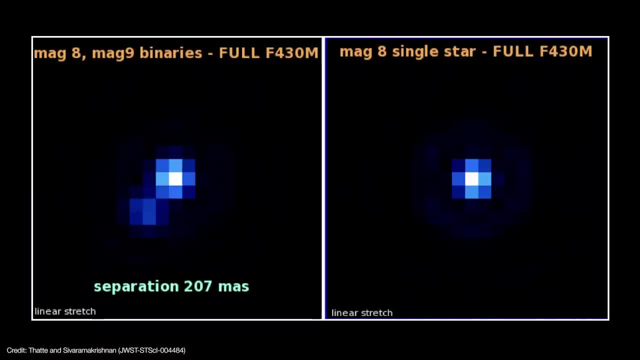 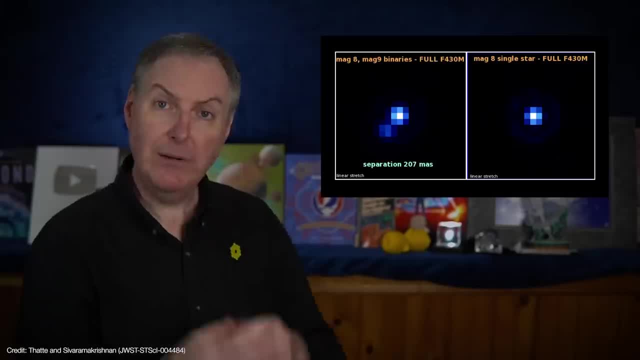 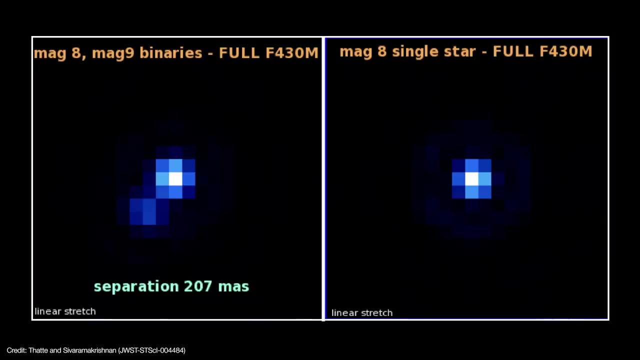 At this scale, both stars in the system are just blocks of pixels. But which pixels correspond to the actual positions of each star? Well, the two stars are too close together for Webb's coronagraphs to be of any use. But when NIRIS operates in AMI mode? 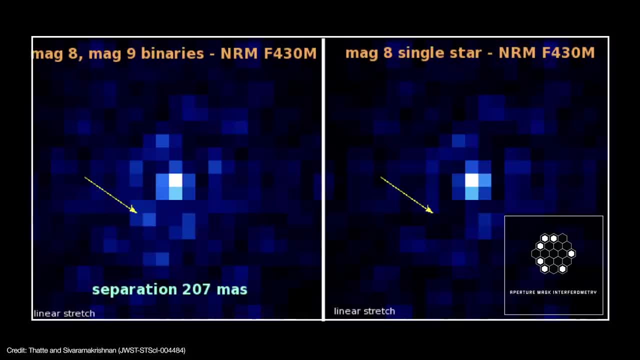 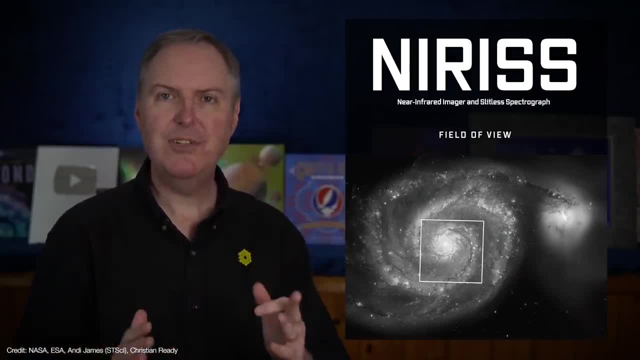 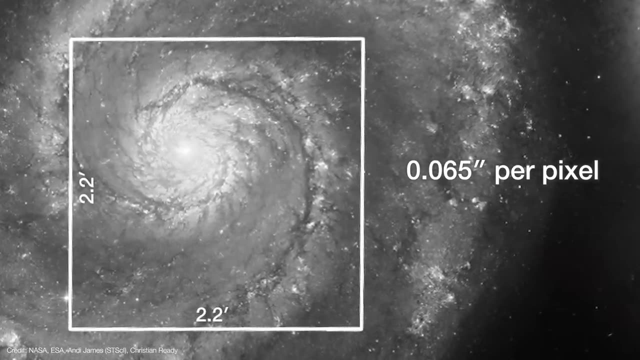 the exact position of the companion star is revealed. And finally, NIRIS's imaging mode allows high-resolution multi-wavelength imaging over its entire field of view, That's, with an imaging resolution of just 0.065 arc second per pixel, And it can operate as a second. 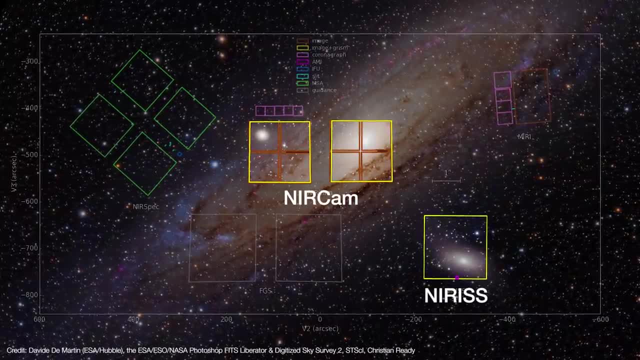 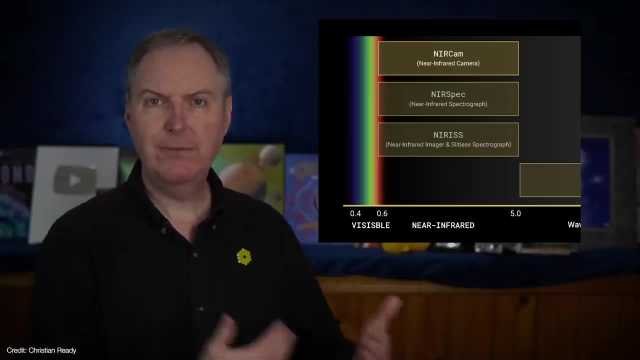 or technically, a third camera in parallel with NIRCam. Not bad for a spectrograph. NIRCam, NIRSpec and NIRIS are all near-infrared instruments, so they're sensitive from around 0.6 to about 5 microns. 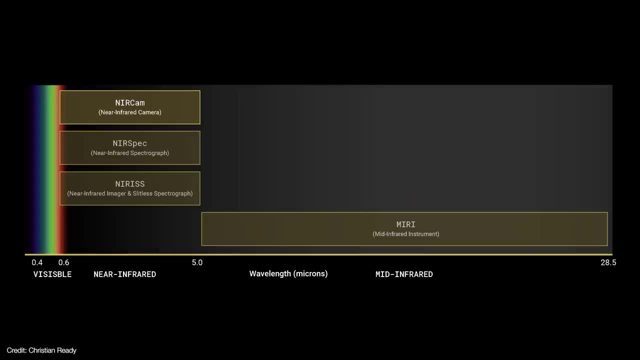 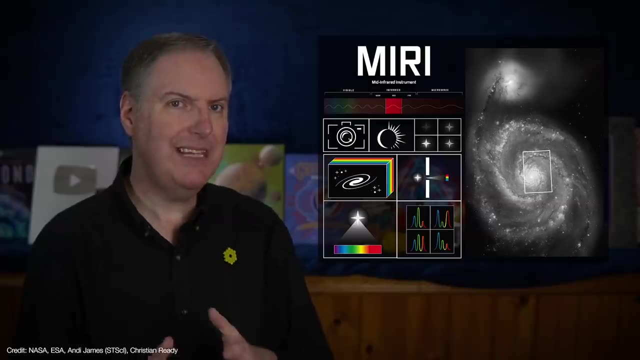 But the mid-infrared instrument, or MIRI, picks up where the others leave off and continues all the way out to 28.5 microns. But looking deeper into the infrared means that MIRI has to be even colder than its near-infrared siblings. 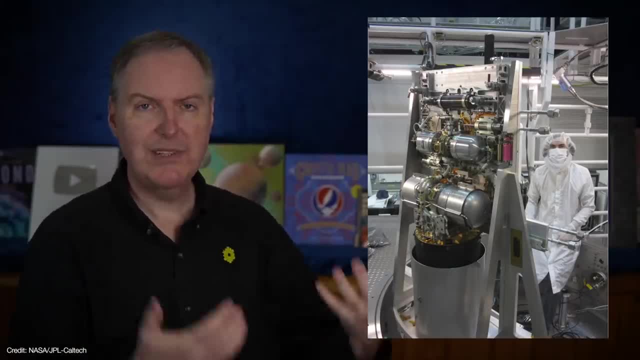 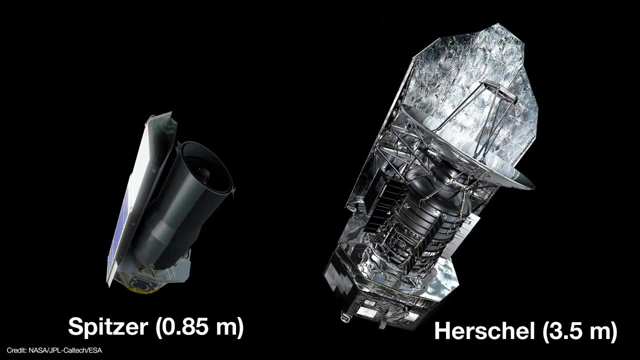 So that's why MIRI uses a cryo-cooler to bring its temperature all the way down to less than 7 degrees above absolute zero. Previous spacecraft like Spitzer and Herschel used liquid helium cryostats to bring their instruments down. 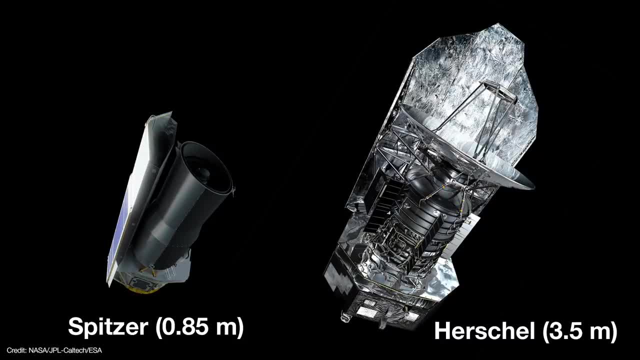 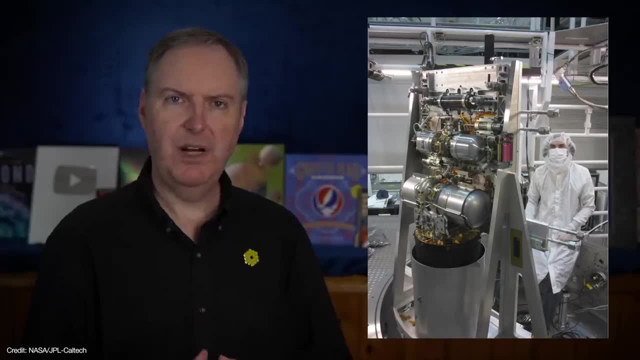 to similar temperatures. As the liquid helium boils off, it carries away heat, But once all the liquid helium is gone, the instruments warm up. MIRI avoids this problem with a first-of-its-kind four-staged closed-cycle cooling system. 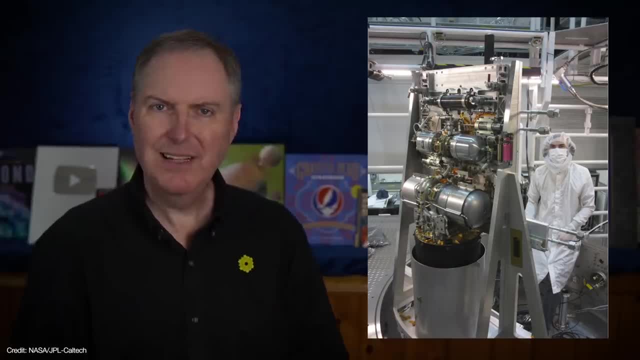 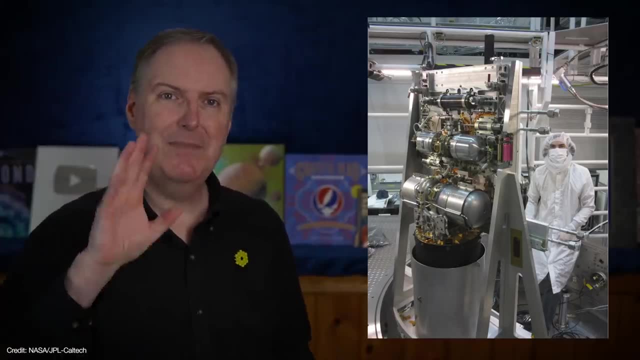 In other words, a killer refrigerator. I'd love to nerd out on just the cryo-cooler alone, but I know this video is getting a bit long. But the point is is that MIRI's lifespan is not limited by any expendable cryogen. 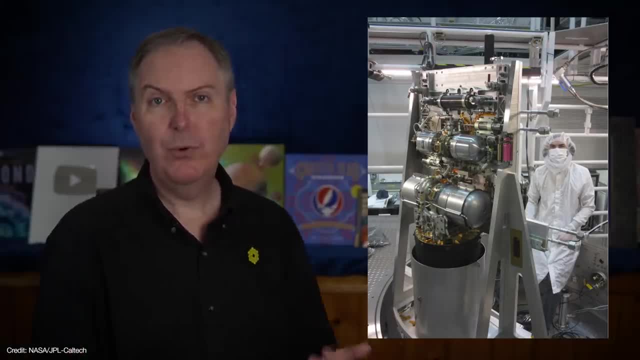 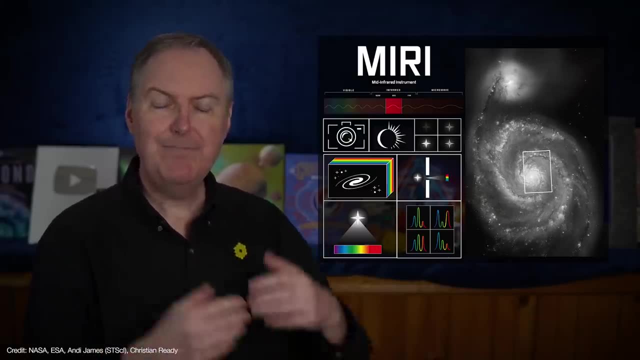 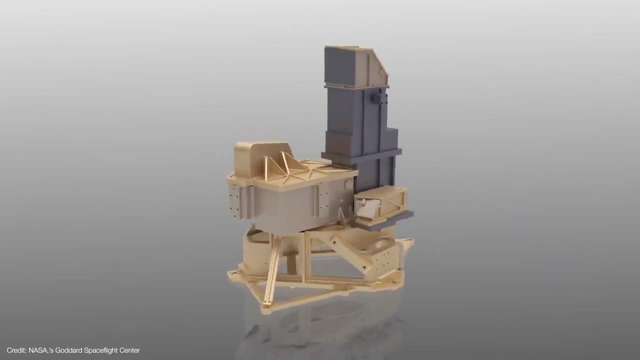 So it should continue to operate for the duration of the mission. Because MIRI is Webb's only mid-infrared instrument, it basically does a little bit of everything else that the other instruments can do. To that end, MIRI is physically set up. 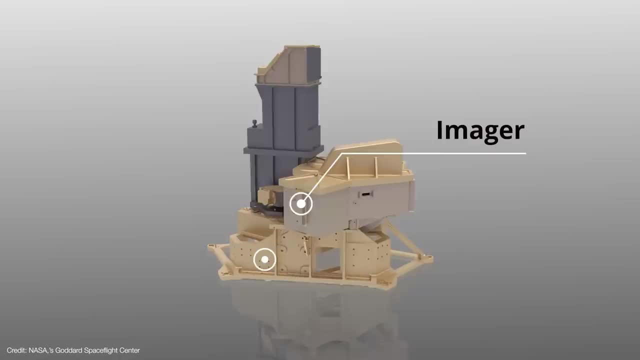 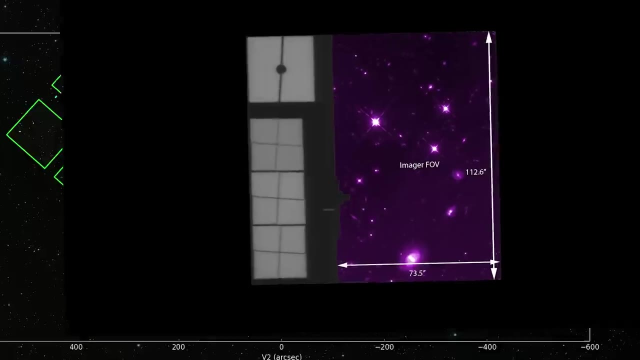 so that one half of the instrument handles the imaging and the other half handles the spectroscopy. MIRI's imaging field of view takes up the largest section of its focal plane. It gets a resolution of about 0.11 arcseconds per pixel. 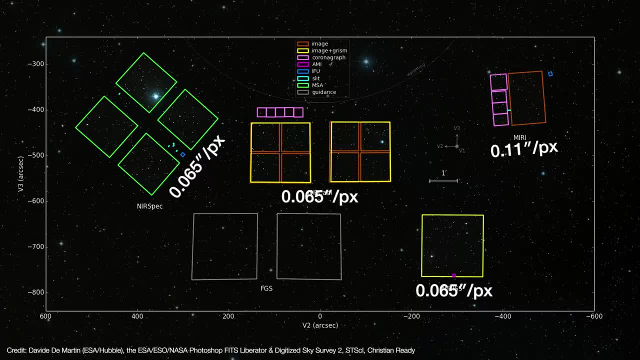 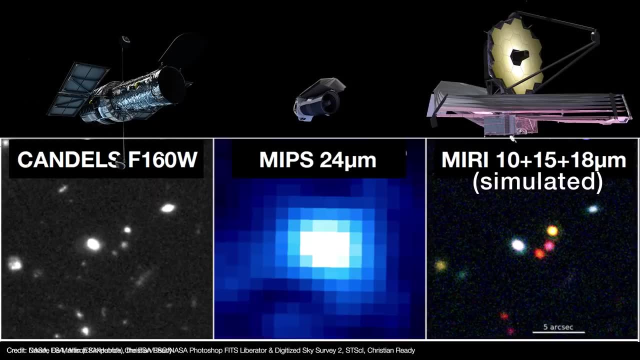 Now that's about half of NIRCam and NIRis's resolution. But we have to remember that the longer the wavelength, the lower the resolution gets. Still, with a 6.5 meter primary mirror, MIRI achieves a much sharper resolution. 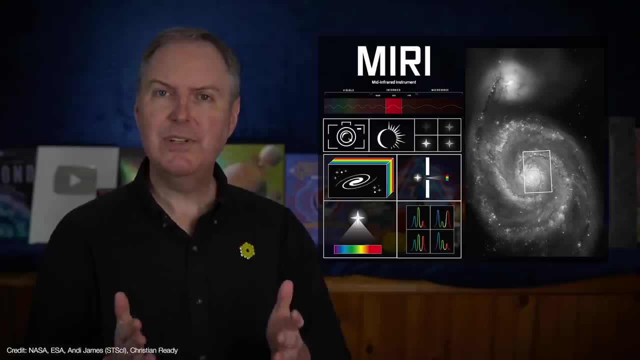 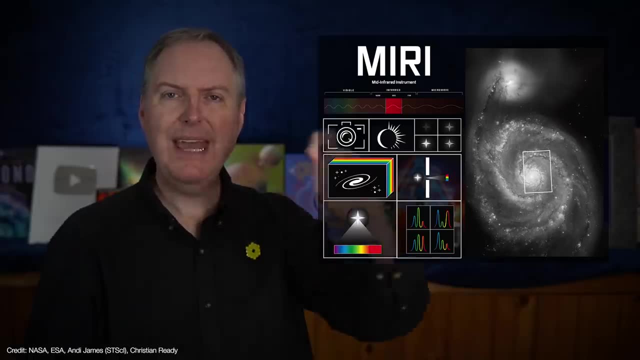 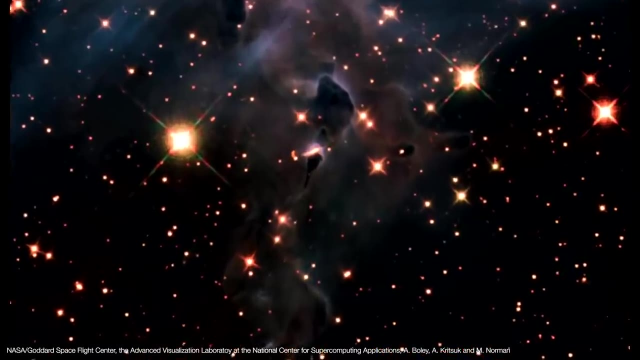 than Spitzer ever could. But resolution is only half the story. Just by virtue of seeing deeper into the mid-infrared, MIRI will be able to look through even more dust and gas to reveal the interiors of stellar nurseries. It will be our clearest look yet. 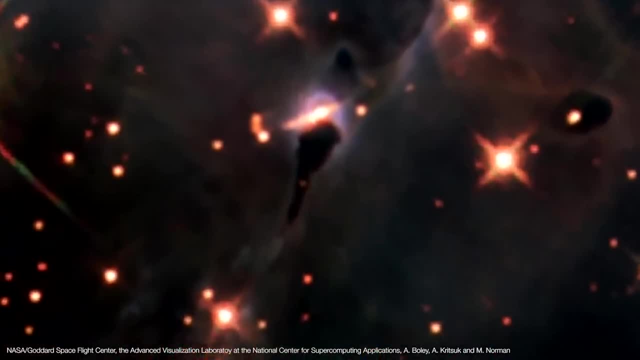 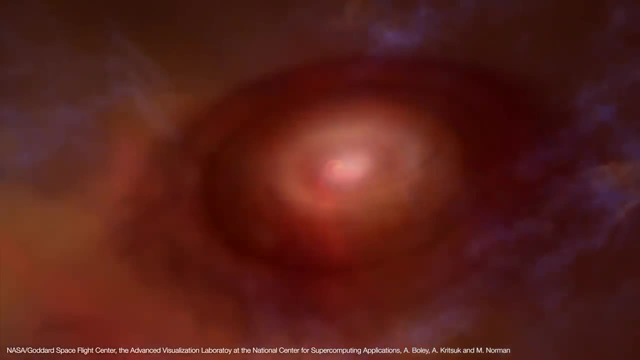 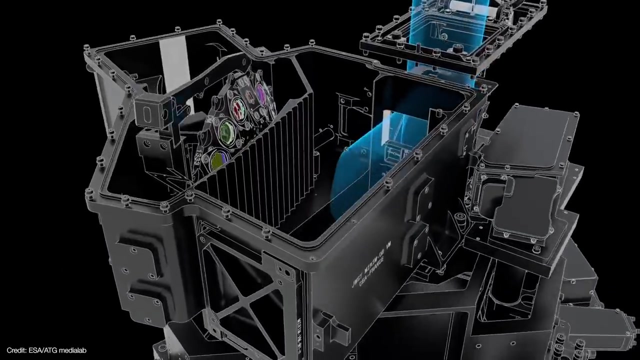 at watching embryonic stars forming inside their dusty cocoons. It's also going to be a great camera for imaging icy bodies in the Kuiper belt and understanding how our solar system formed. The optical system of the camera consists of five mirrors and a filter wheel. 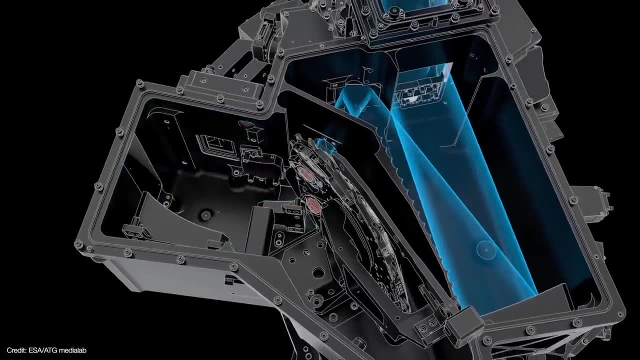 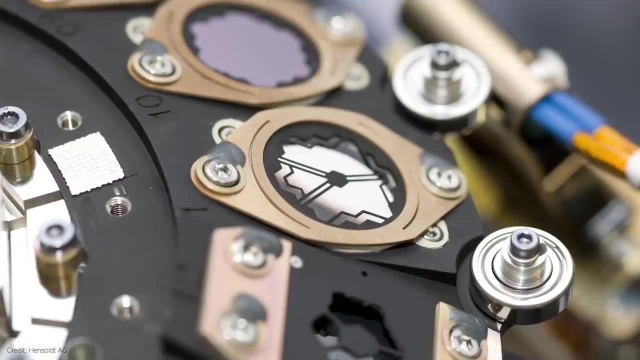 The wheel consists of 18 elements, nine of which are filters for wideband imaging, But the wheel also has four coronagraphic imaging filters as well, And these are special filters that combine with MIRI's coronagraph masks to block out a star. 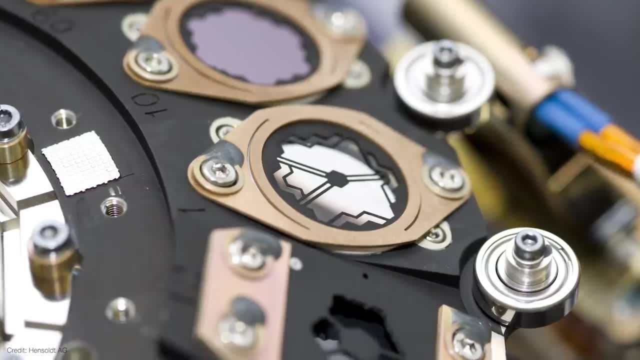 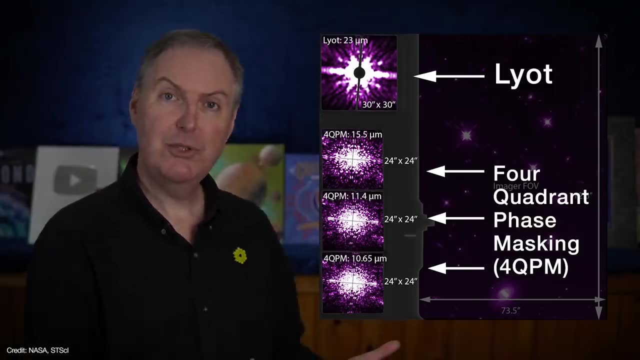 and let MIRI directly image the surrounding planets. There's actually two kinds of coronagraphy that MIRI supports. There's the traditional mode called a LIOT coronagraph, which places a small circular mask that's suspended by a bar and blocks out the star. 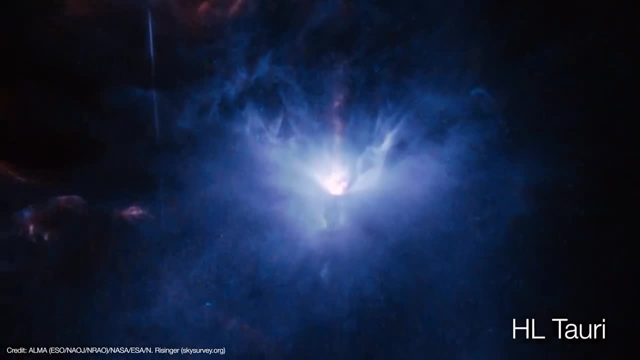 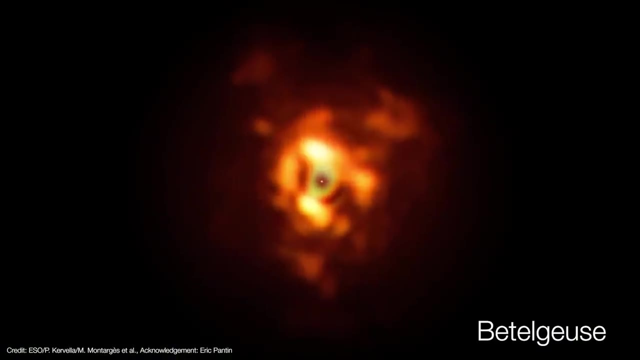 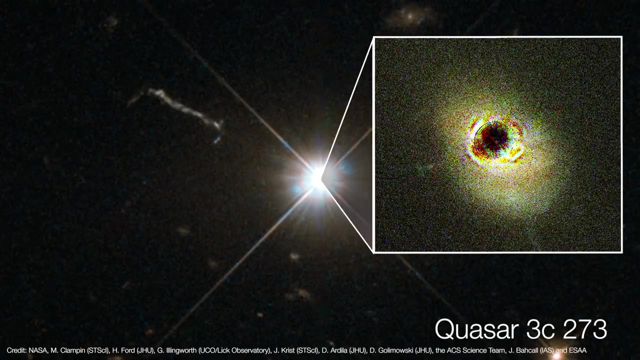 And this approach works well for investigating diffuse objects near bright sources, So for example the outer regions of a protoplanetary disk, the ejected dust cloud around old dying stars or the central regions of active galactic nuclei. But the mask always imposes a limit. 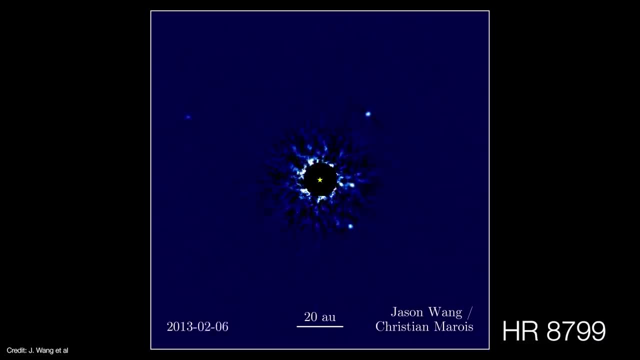 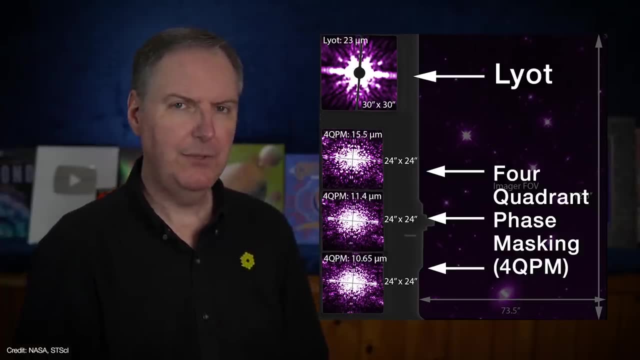 on just how close you can get to the star, And that's why MIRI allows for a new kind of coronagraphy called four-quadrant phase masking or 4QPM. It's a special mask that splits the field into four quadrants. 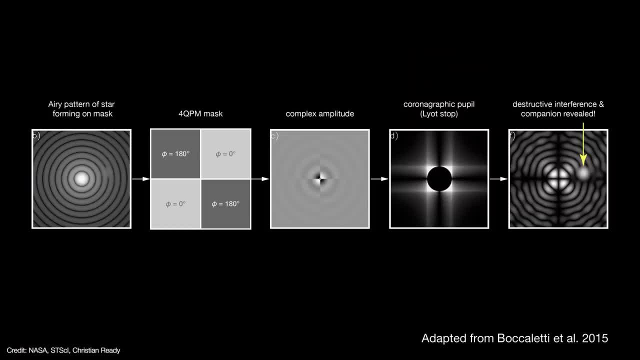 Light waves passing through two of the quadrants are shifted 180 degrees out of phase with the waves passing through the other two. The two sets of waves destructively interfere and cancel each other out. This lets MIRI study exoplanets that are up to three times. 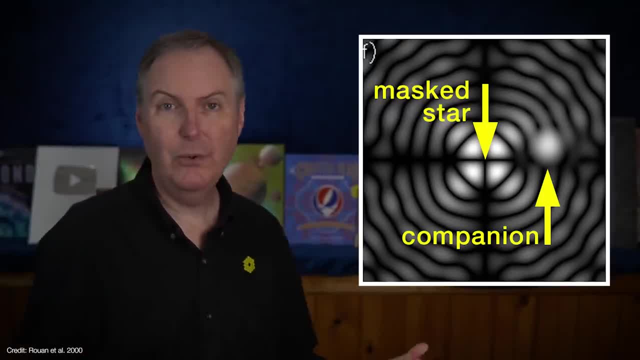 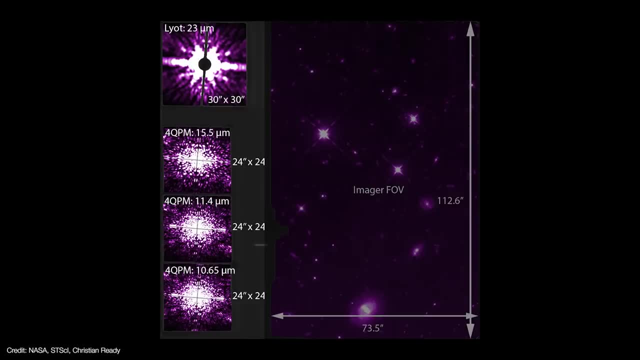 closer to their host stars than it could with the old-school Lyot coronagraph. And there's actually three different 4PQM masks, each of which are optimized for a different wavelength of infrared light. But all of that is just half of what MIRI can do. 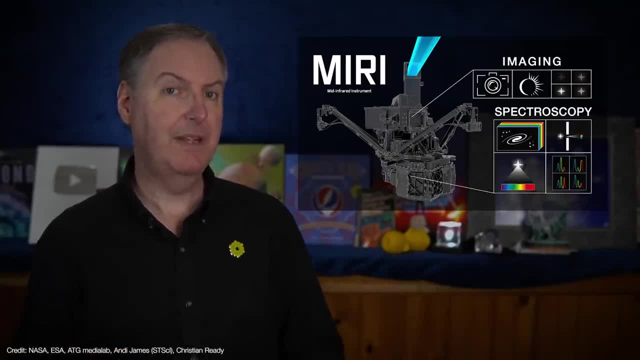 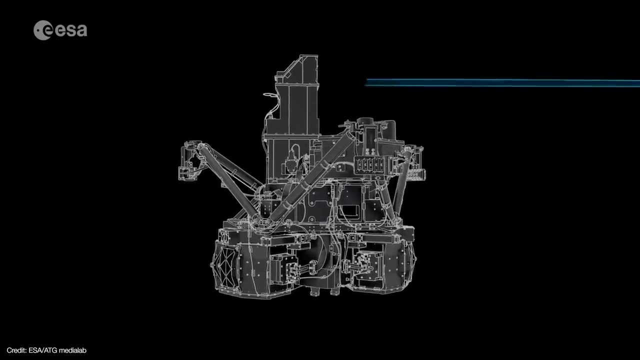 The top half. to be precise, The bottom half of the instrument houses MIRI's medium resolution spectrograph. Initially, light enters through the top half of the instrument where the imaging hardware is located. After passing through the initial formatting mirrors, the beam is sent to the bottom. 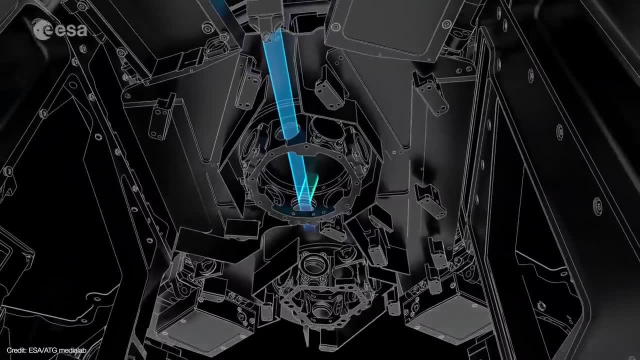 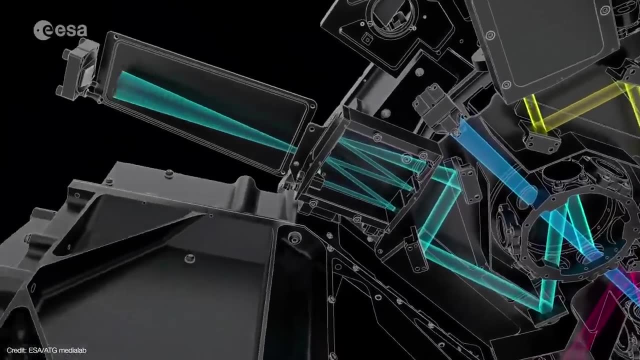 where the spectrograph is located. After light enters the spectrograph, it is split out into four channels, each of which are sensitive to different parts of the spectrum. The image is sliced into segments, which are then fed into a maze of relay mirrors and grisms. 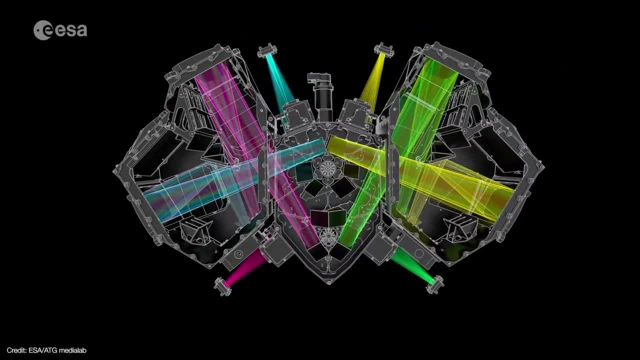 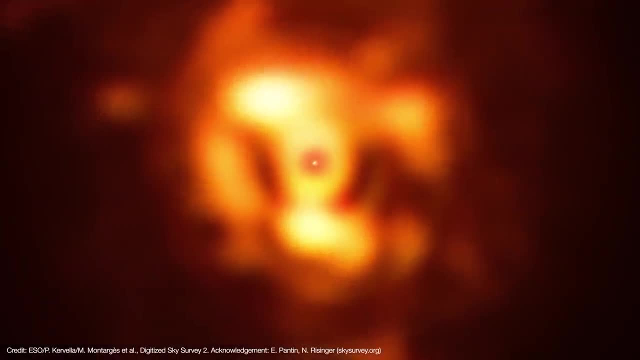 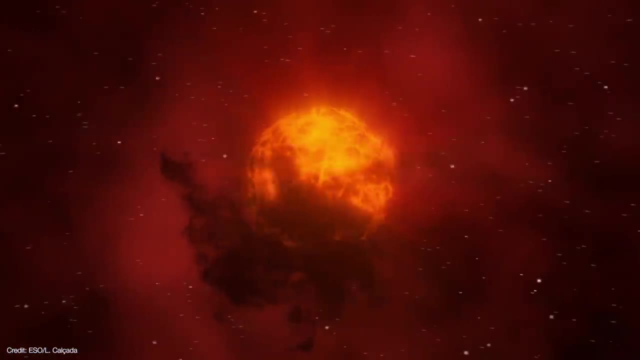 that disperse the image into a final spectrum. The result is that MIRI will see through the surrounding dust belched out by evolved supergiant stars and take the spectrum of the water forming in their convulsing atmospheres, Or perhaps understand how the ejecta 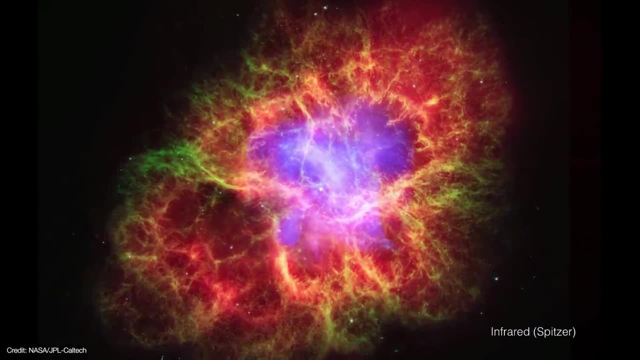 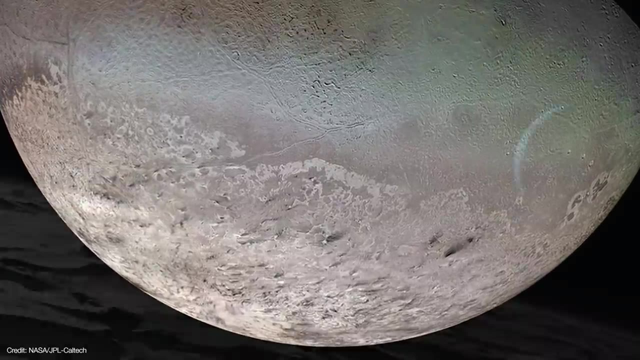 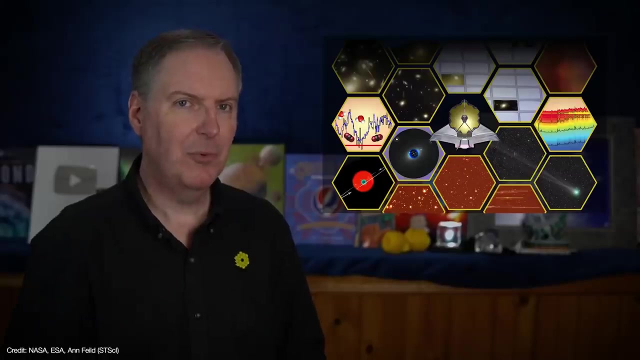 from supernovae, interact with the interstellar medium to produce new stars, Or even investigate the cryovolcanoes of Neptune's moon Triton and understand how they contribute to its atmosphere. If a picture is worth a thousand words, spectra are worth a thousand pictures. 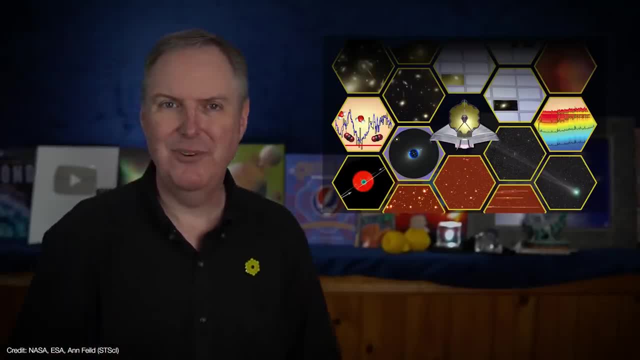 And Webb is going to give us so many of both Now. I know I've said this before, but the skills required to just design and build these instruments is nothing short of mind-blowing. The good news, though, is that skills can be learned.